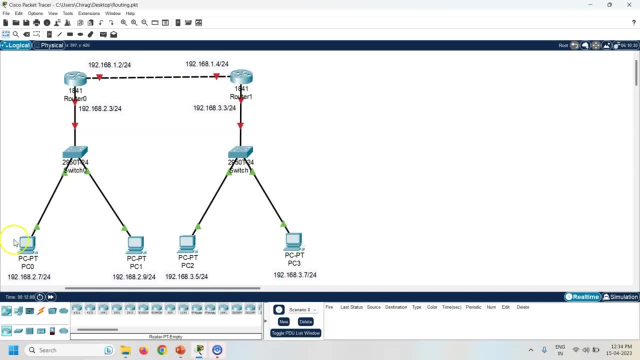 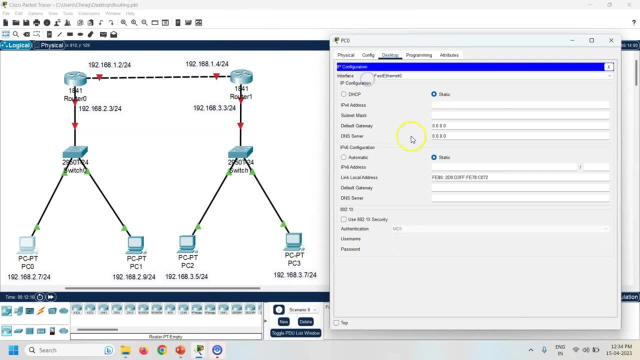 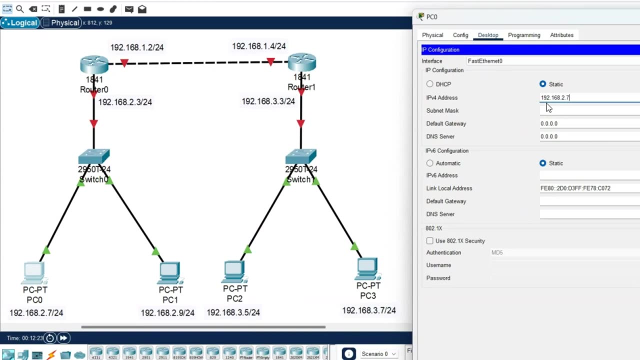 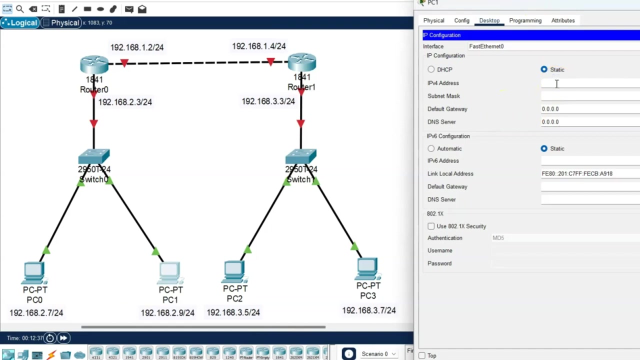 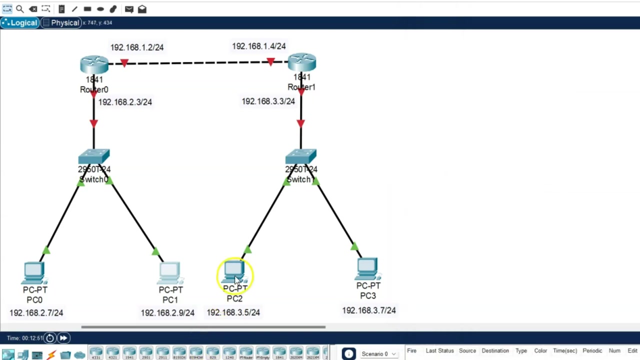 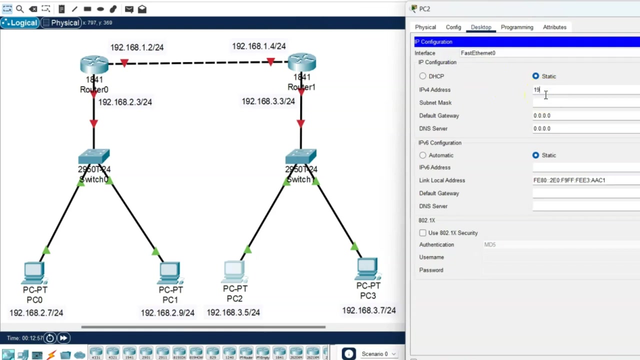 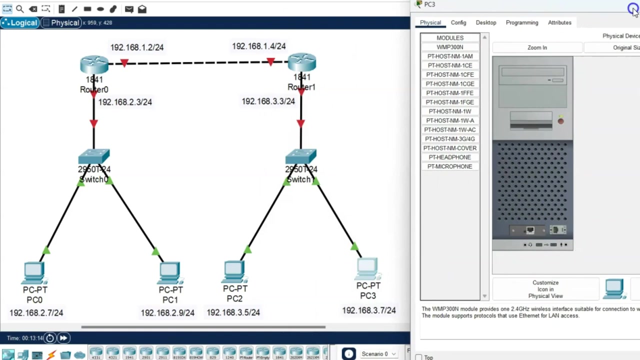 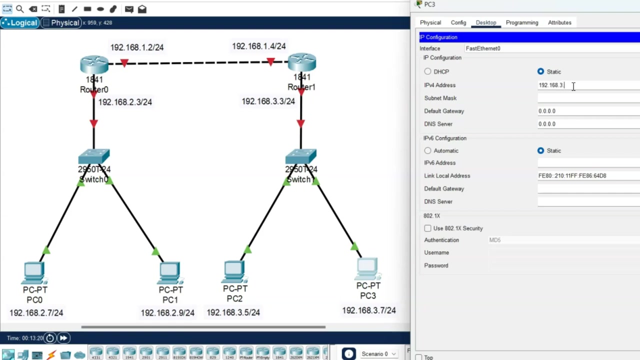 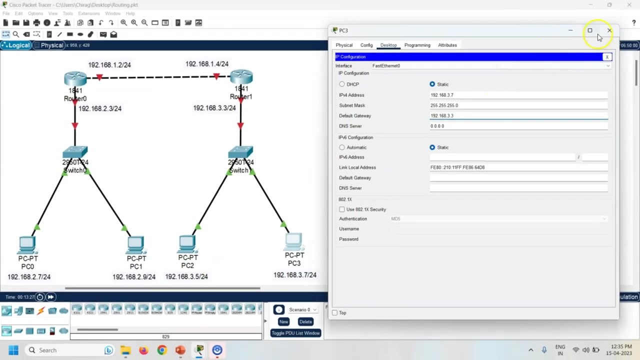 Now assign the IP address to all the PCs as per the given label. Next, set up the IP address of the system and the IP address of the PC. Set up the IP address of the system as per the given label. next task is assign the IP address to the router interface. now check the interface. so. 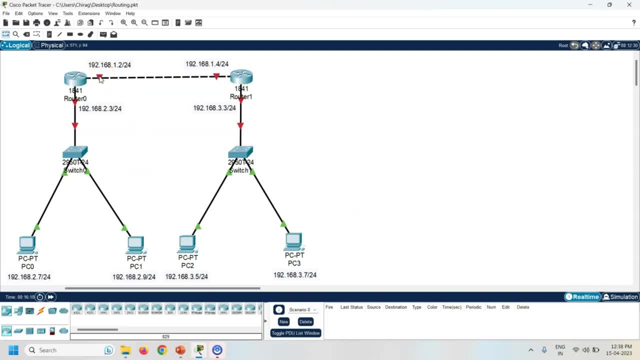 here. both the routers are connected with the fast ethernet 0: 0 interfaces. so same way, check the other interface of the router. it is FH 0- 1 which is connected with switch. same way, check into the router 1. now router 1. other interface is FH 0: 1 which is connected with the switch. now click on. 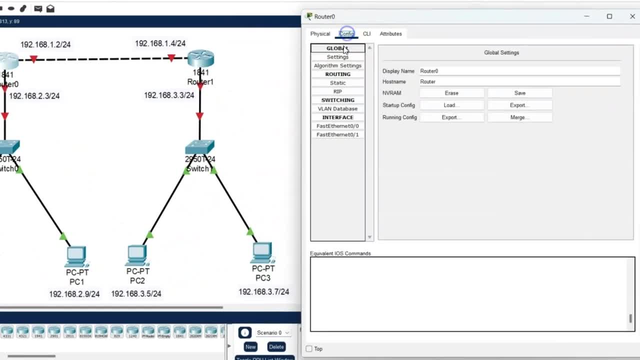 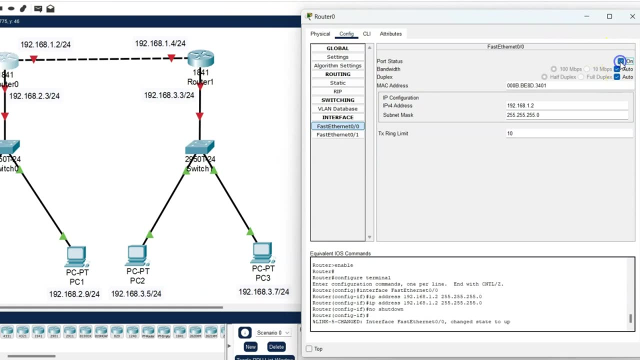 the router. go to the config, click on the fast ethernet 0- 0. the IP address is 192 dot 168 and dot 1 dot 2. now. port status is on. now click on the fast ethernet 0- 1. the IP address is 192 dot. 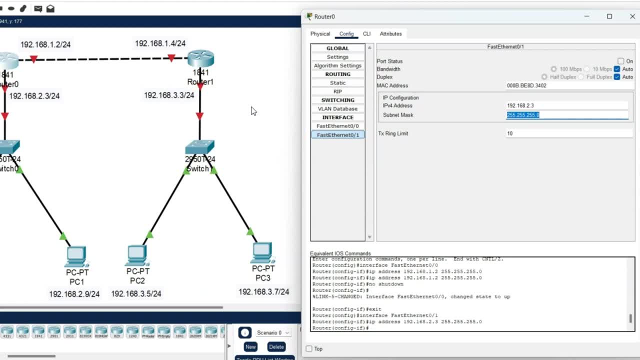 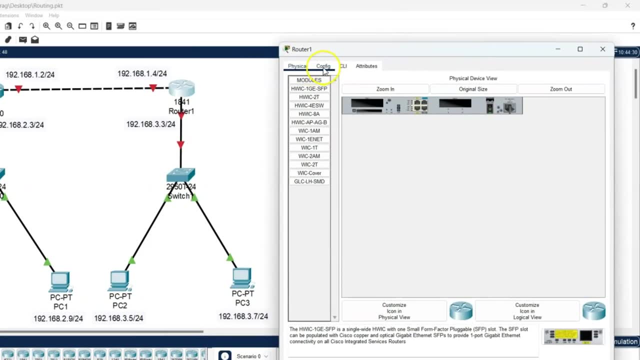 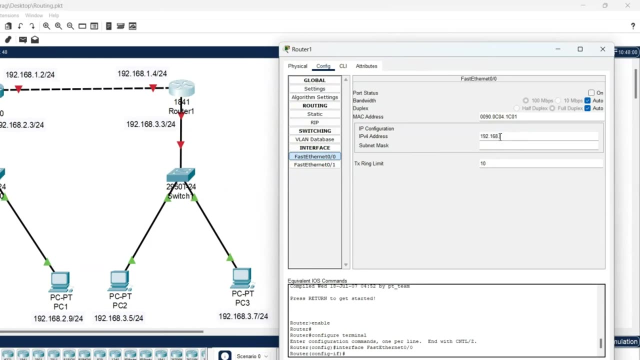 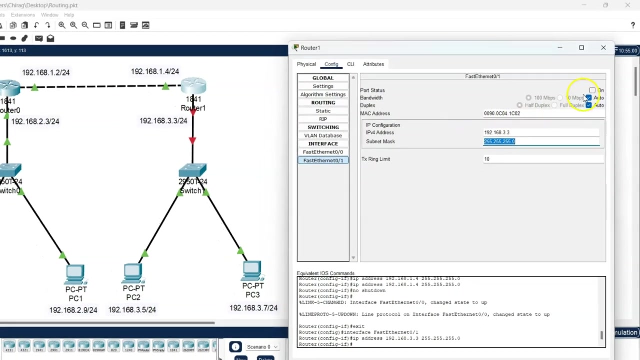 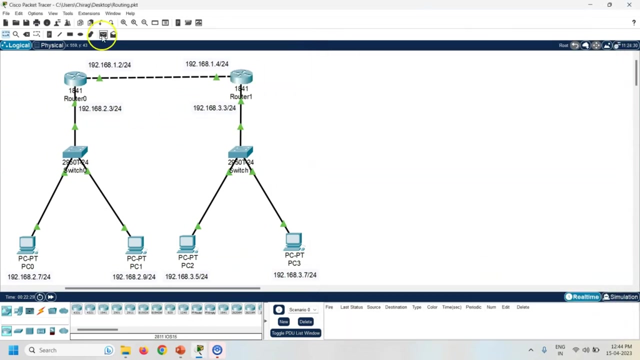 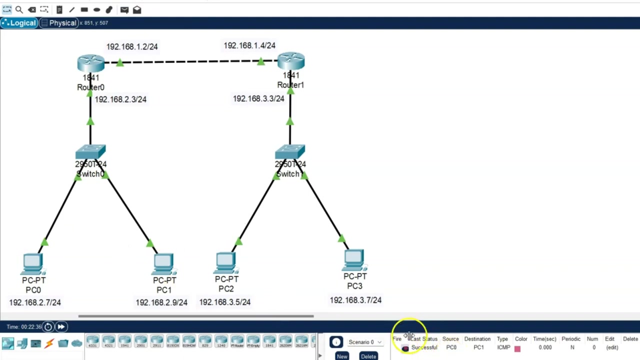 168, dot 2, dot 3. again, port status is on. so now same way: configure the router 1. next task is check the connectivity between all the pieces. so take one simple PDU: click on the source and PC 1 is the destination. now you can check here. it is successfully transferred. 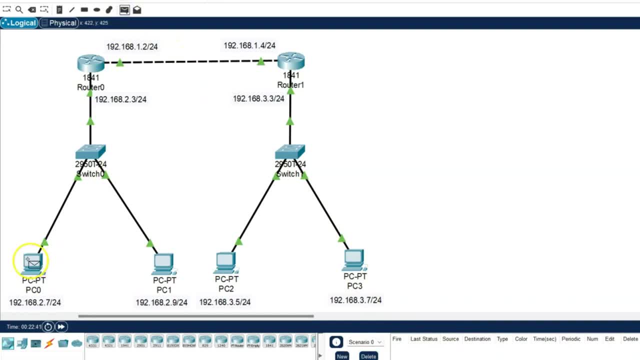 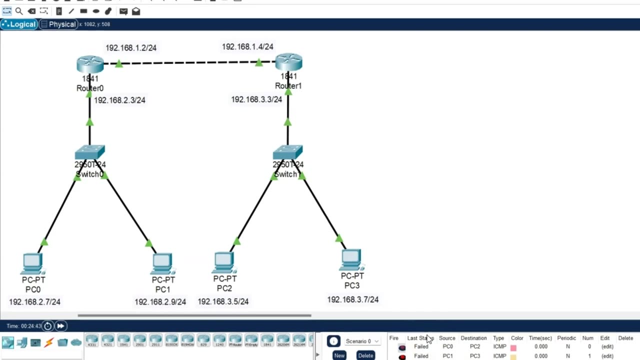 now again. take one simple PDU: PC 0 is the source and PC 2 is the destination. so it is failed. now same way, take another simple PDU: PC 1 is the source and PC 3 is the destination. again it is failed. so now we can say: PC 0 and PC 1 are in the same network and PC 2 and PC 3 are in the different. 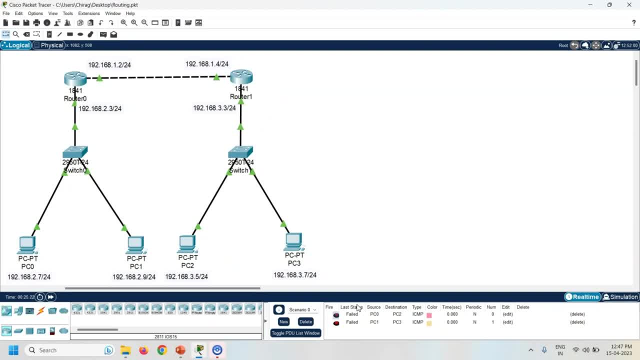 network. if I want to communicate with the different network pieces, I have to configure a routing. so what is routing? routing is a process of selecting a path to transfer the data from source to destination. so there are two types of routing: one is the static and second one is the dynamic. here, 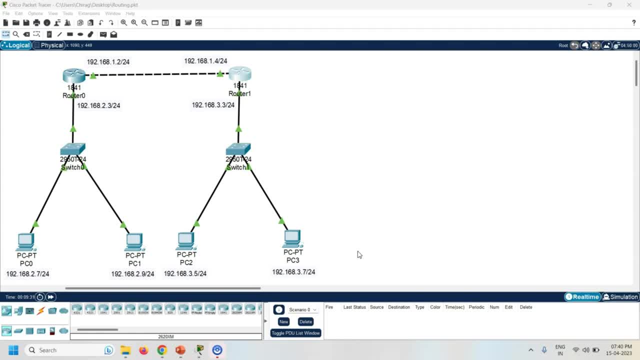 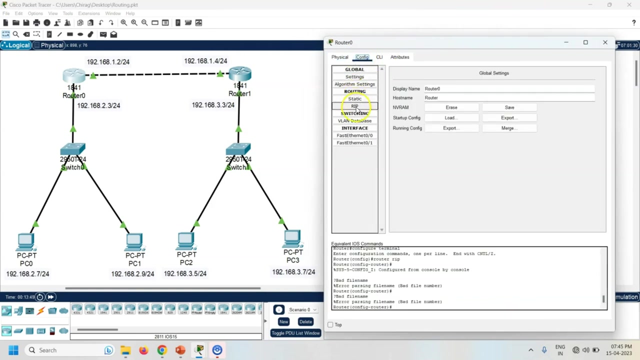 I am going to configure dynamic routing on both the routers. so first of all, what is dynamic routing? dynamic routing uses algorithms to determine the best path. examples of the dynamic routing are rip. so first of all, click on the router 0, go to the config, click on the rip. rip stands for routing. 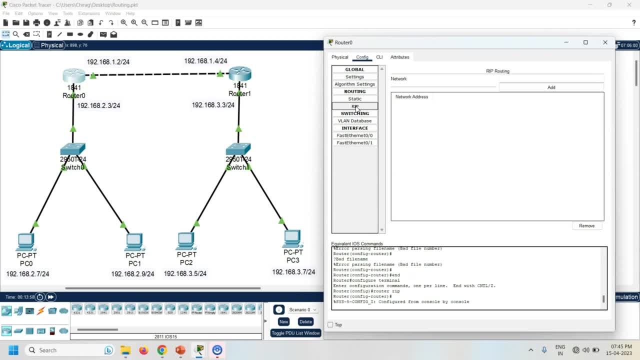 information protocol. it is one kind of dynamic routing algorithm. here router 0 is connected with 1.0 and 2.0 network. so here I am adding both the network address. so first of all I have add 192.168.1.0. then click on the add button so it is added over here now at the next network address- it is 192.168.2.0- and add in the list. so now both the network address are added in the list. now go to the setting and click on the save button. 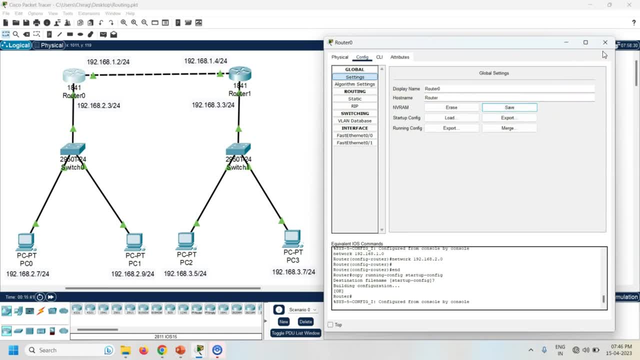 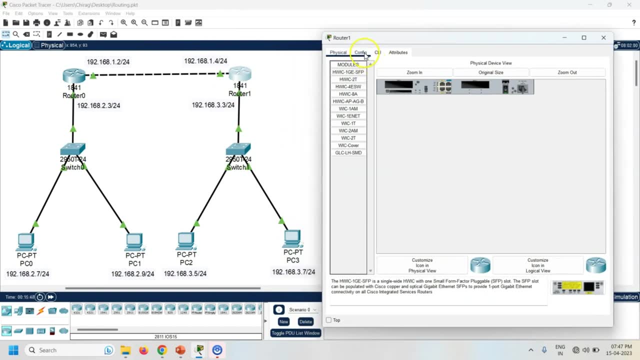 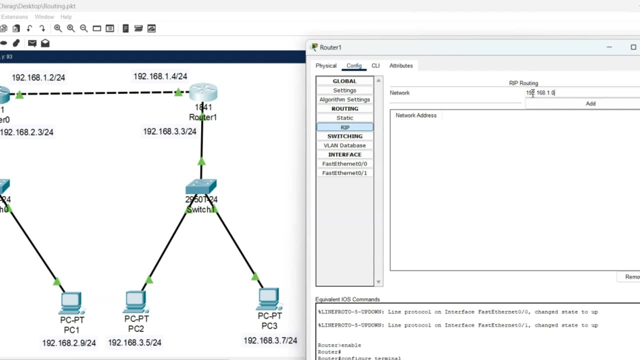 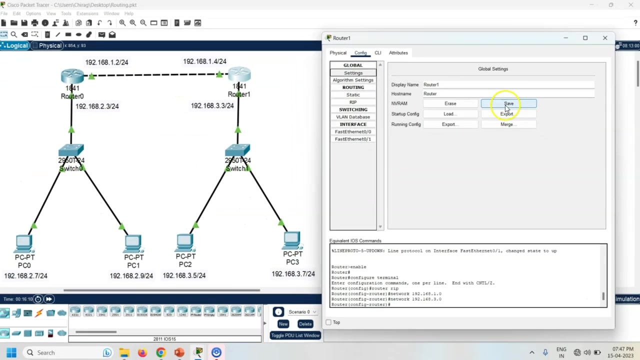 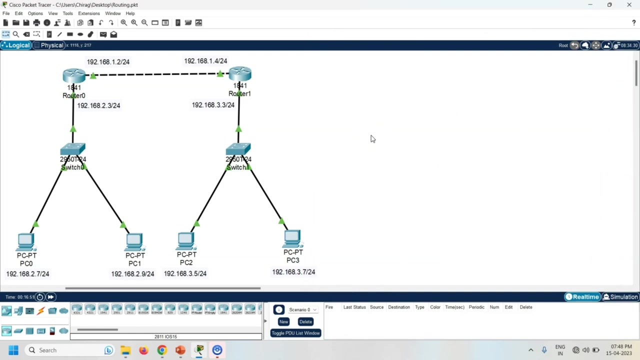 to save these changes in the startup configuration of router. now, same way, configure the router one. so now watch some video onаныib router. aye, so now my both the routers are configured. let's check the connectivity of PC2 and PC3 from PC0.